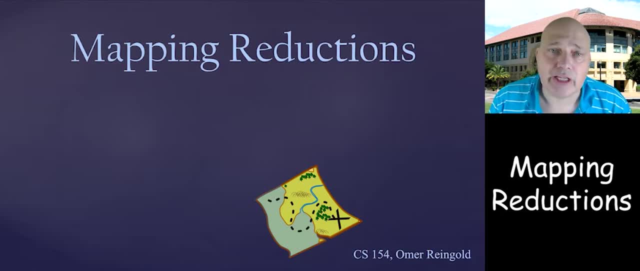 these other problems are also not decidable or not recognizable depending on the problem. So reductions are kind of the maybe one of the major techniques- if not the major techniques- we're seeing in this class, And we're seeing it in a way which is opposite to the algorithmic. 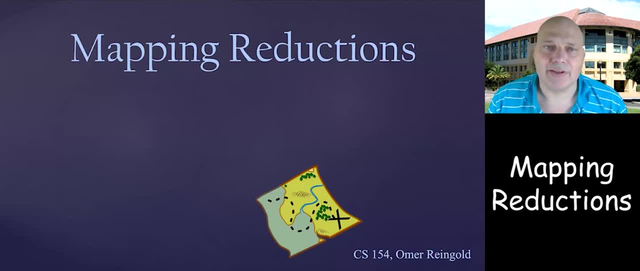 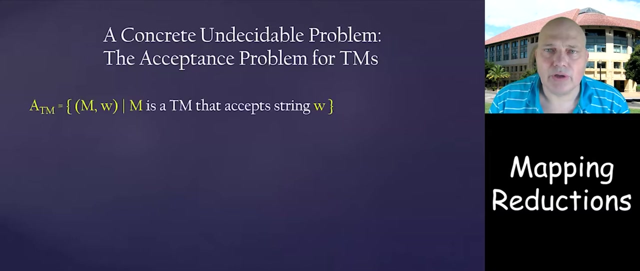 rhythmic manner of using reductions to solve something. Here we're using reductions to show that something is impossible, And this is something we'll meet again when we'll talk about complexity. We'll see reduction to show that something cannot be done efficiently. So our concrete problem was ATM. We showed that ATM is not recognizable, So it's recognizable. 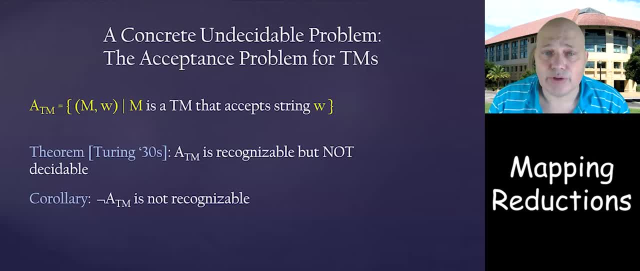 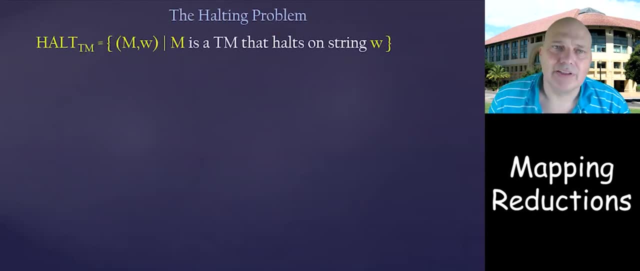 but not decidable, And the corollary showed that not ATM is not recognizable. Let's look at the second problem, the halting problem. The halting problem also is a language over pairs M, which is a Turing machine, and W, which is string, And these are pairs where M 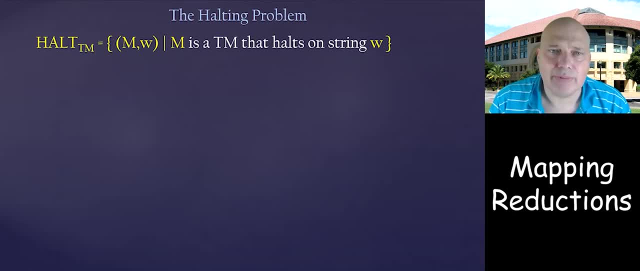 is a Turing machine that halts on string W. So in ATM we wanted M to halt and accept W, but in halting we only care that M halts on W. This is definitely something we want to know. I mean, we would love not to run algorithms that run into a loop. So before running the algorithm, 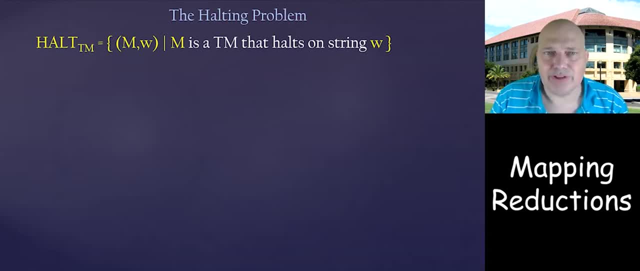 we can check that it's going to stop. This would be a positive thing, And the theory is that HALT is undecidable. Let's see a proof. Assume, for the sake of contradiction, you have W at h, you have A at L at H and you have W at A at H, You have W to the enclosing thought. In addition, there's 1 minus A, So this is saved, theHIM delicacy. this is the method of constipation of H. Now you have W and you have aniszt sellers andlev toujours que os 로comb, Y'all filling ends. 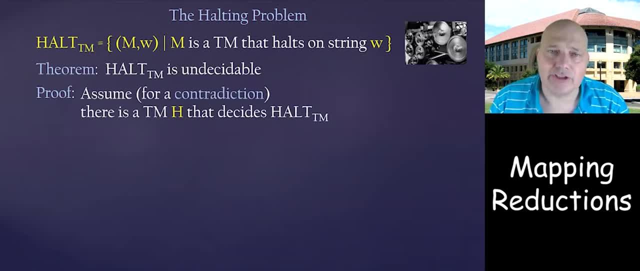 for the sake of contradiction, that there is a Turing machine H that decides Alt-tm And we're going to use H to construct a Turing machine M prime that decides A-tm. This, of course, is going to be a contradiction, because there is no Turing machine M prime that 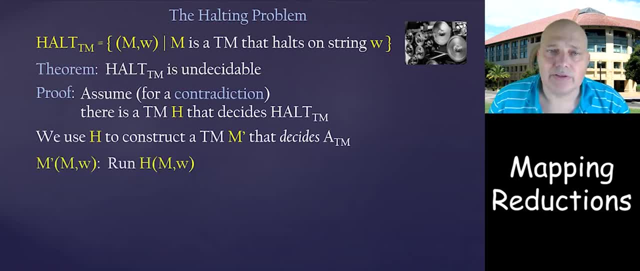 decides A-tm. So let's see how we're going to run, how we're going to define M prime. So M prime is a machine that is supposed to decide A-tm. The way it will do it, it will first run H on M w. 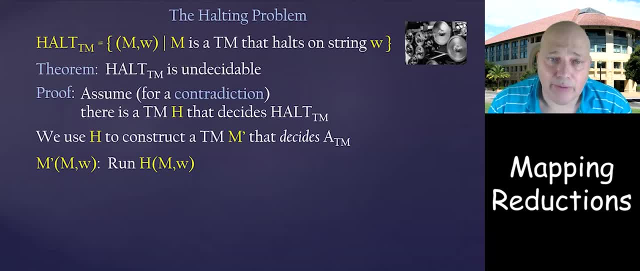 H is the machine that tells me if M halts on w. If H rejects, it means that M is not going to halt on w and definitely it's not going to accept. so M prime can also reject If H accepts. then we can safely run M on w. 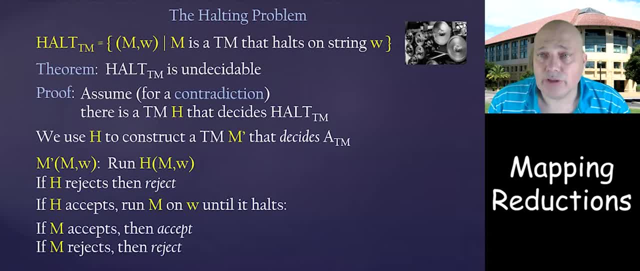 because it's going to halt. And when it halts, we can output what M does. If M accepts, we're going to accept, If M rejects, we're going to reject. But this simulation is going to surely stop, surely going to halt because M w is in halting. 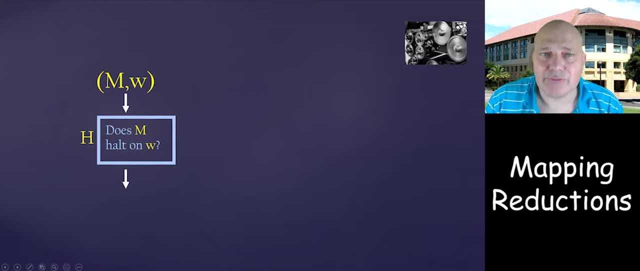 Pictorially what we have. we have this machine M. so this machine H that decides halting it gets an input M, w and it's going to tell us if M halts on w. We're going to take this machine and use it as a subroutine within a bigger machine that. 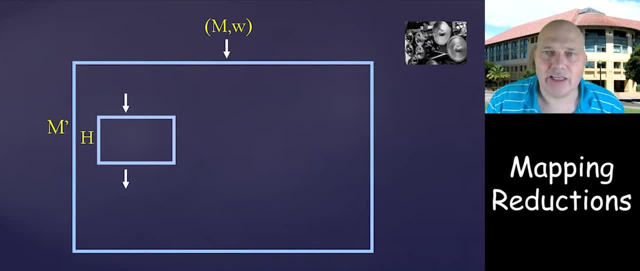 is going to decide for us A-tm. So the input for A-tm is M, w. We're going to feed it first to our subroutine H and C. If M doesn't halt, then we can reject, because we know that M definitely doesn't accept. If it doesn't halt, it doesn't accept. And if M halts then we can feed it. 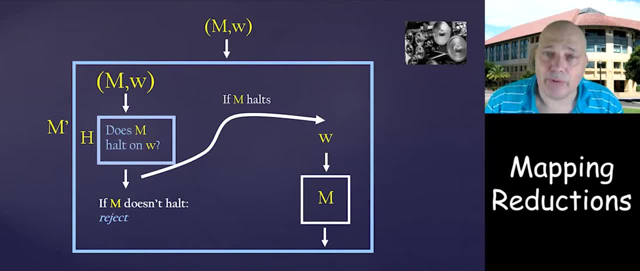 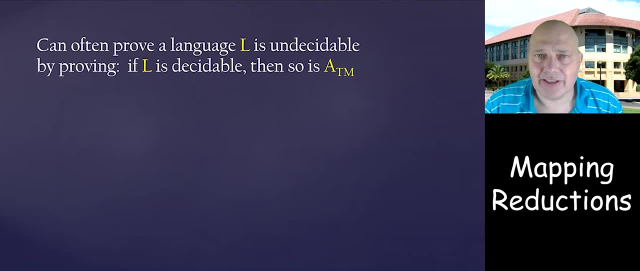 to M itself, And so we feed w to M and we output whatever there is to output. So this is kind of we can. actually there is a proof that halting is undecidable just by a diagonalization argument pretty similar to the one we saw for A-tm. 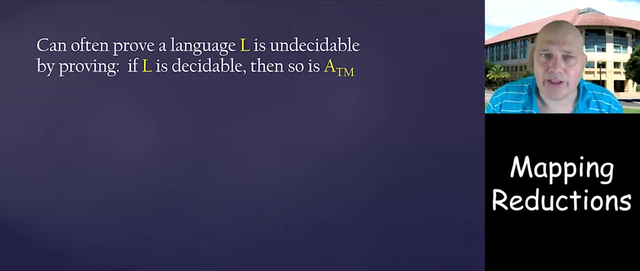 But instead of having two of these arguments here, we did it directly, And we can often do something like this. We can often prove that the language L is undecidable by showing that if L is decidable, then so is ATM Meaning. we show a reduction from ATM to L. 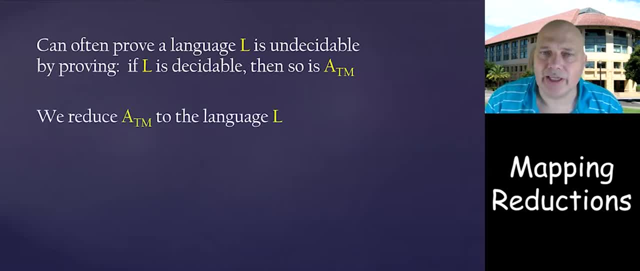 We reduce ATM to the language L and we'll call this: ATM is smaller, equal M, L Or, in words, ATM is mapping reducible to L. What we saw actually is not a mapping reduction. we'll talk exactly what the mapping reduction is. So what is a mapping? 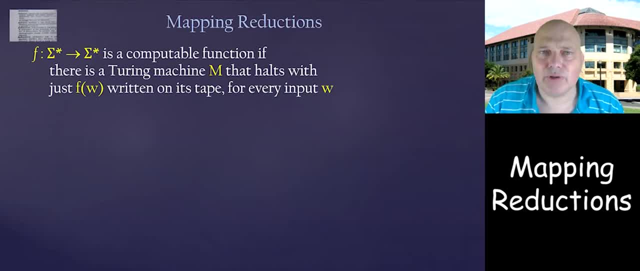 reduction, A mapping reduction, is a function and it is a computable function. So let's discuss what is a computable function? So a function f that takes a string and output a string is computable. and If there is a Turing machine M that always stops when it has the input, 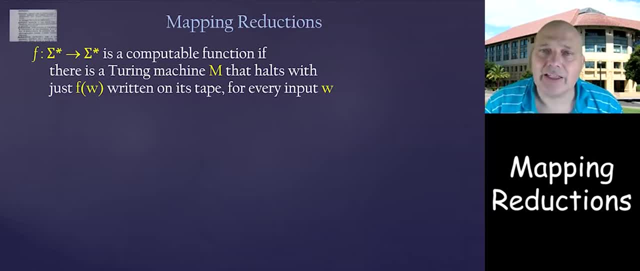 For any input it always halts. And for input W it's going to halt when F of W is written on the tape. So when we wanted to have machines that compute a language, the machine has to just halt and either accept or reject. 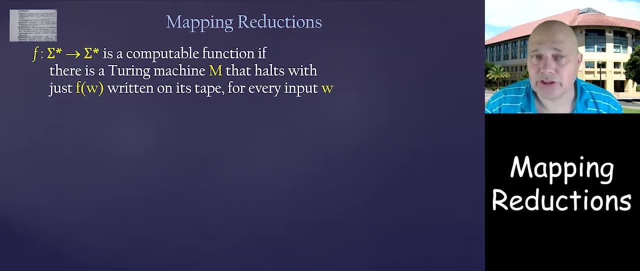 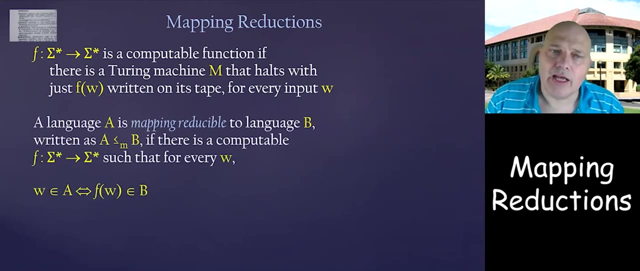 Now we want the machine to halt and write the output, which is F of W. It shouldn't surprise us Any programming that you've done. usually didn't just check if something happens or not, but add some output to it. And now that we have what the computable function is, 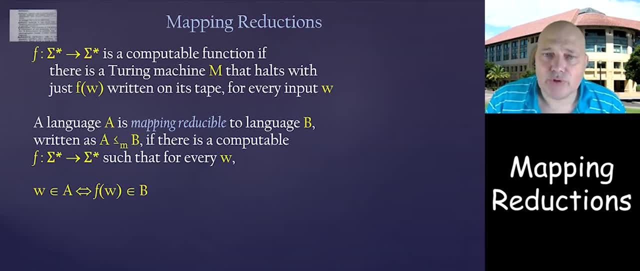 we can say that the language A is mapping, It's being reducible to a language B which will write A smaller or equal M B If there is a computable function F, such that for every W W is in A, if, and only if F of W is in B. 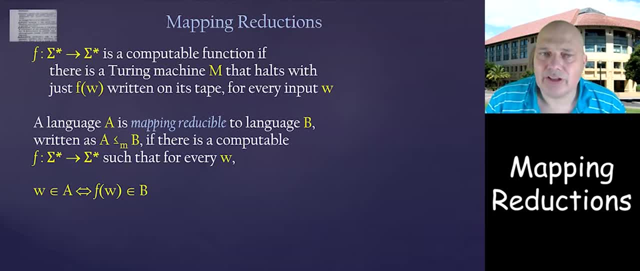 So what does it mean? Why is it a reduction? It's a reduction because, instead of trying to answer if F of W is in A, we can compute F of W and then answer if F of W is in B. And this if and only if W is in A, if and only if F of W is in B. 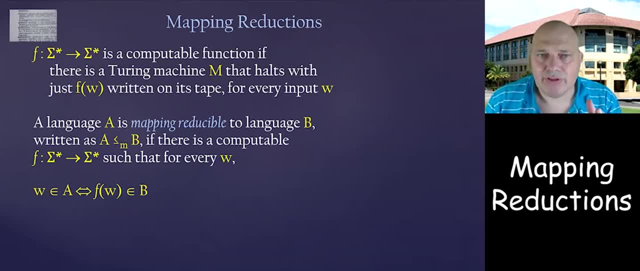 means that solving the problem W in A is exactly the same as solving the problem F of W is in B. So we reduced one problem to the other. We reduced the problem in A, We reduced the problem in B, And that's why we say that A is reducible to B. 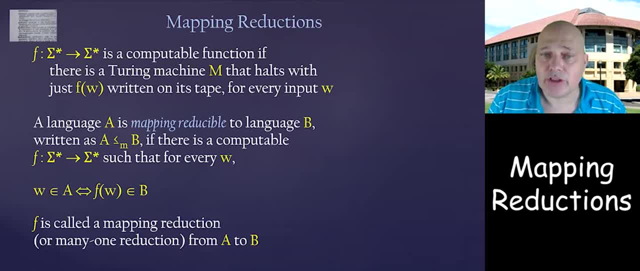 F is called mapping reduction or many-to-one reduction from A to B. It can be many-to-one because nobody says that two different W's cannot map to the same problem. In fact, in some proofs that you'll write, you will have the same. 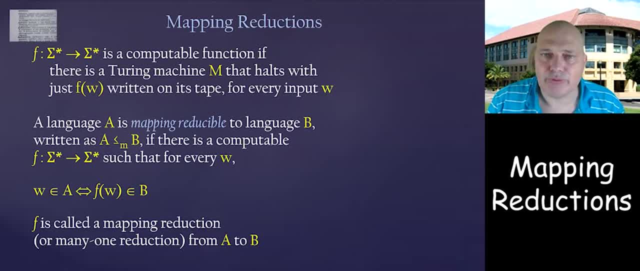 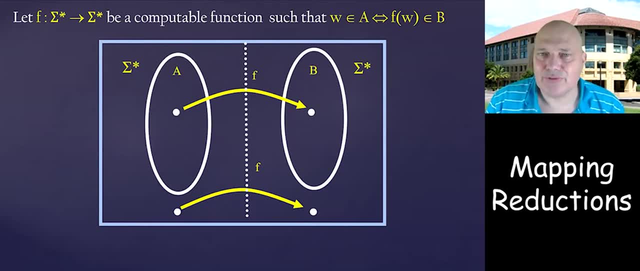 We'll have many, many, many inputs go to the same output. Pictorially, what we have here is a reduction, is a function that goes from strings to strings and the function F, which is computable. You can actually follow these arrows. 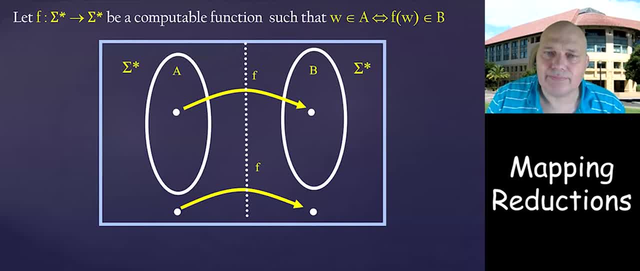 these yellow arrows and such that, such that you have that if you are in A, if you start in A, you end up in B, And if you start outside of A, you end up outside of B. So the question of whether this point that you reach is in B or not in B is exactly the same as the question of whether the original point is in A or not in A. 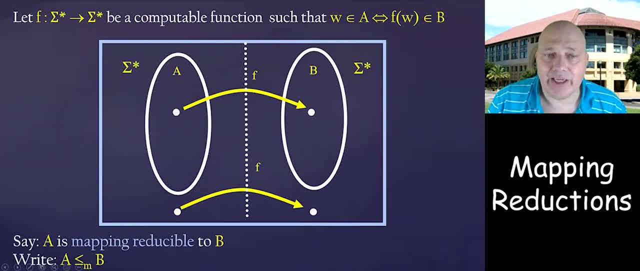 And so we say A is mapping reducible to B and write A smaller equal M to B. And I want you to remember that notation by thinking that A is somehow weaker than B And we'll see exactly why. but that's the way I remember how to write it. 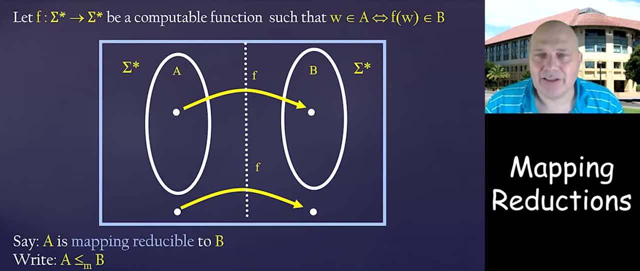 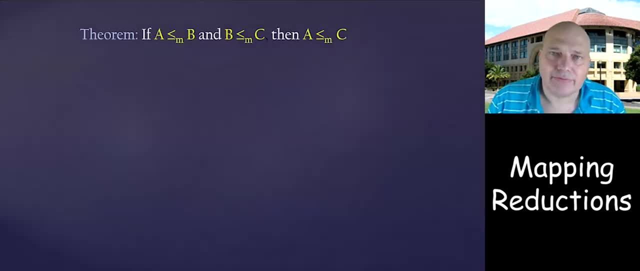 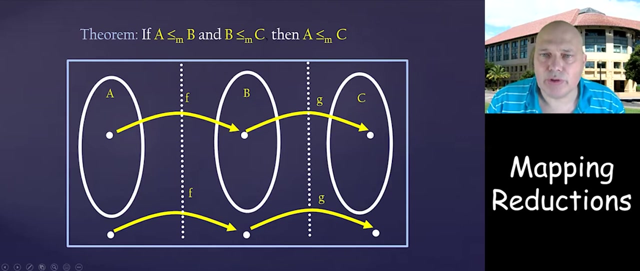 So A reduces to B, It means that it is kind of weaker from B or not stronger than B, And one nice property that we have is transitivity. If A is mapping reducible to B and B is mapping reducible to C, 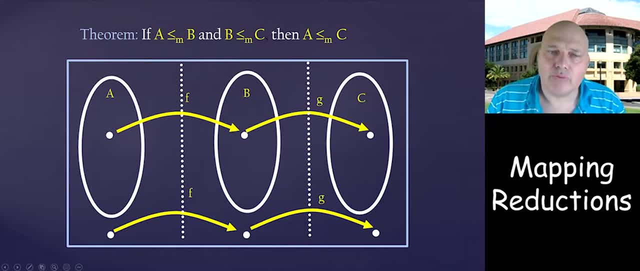 then A is mapping reducible to C And to see that we just need to compose the two reduction to compose F and G, Because to this function it takes you from A, from it applies, first applies A, F and then applies G, and will first be computable because F and G are. 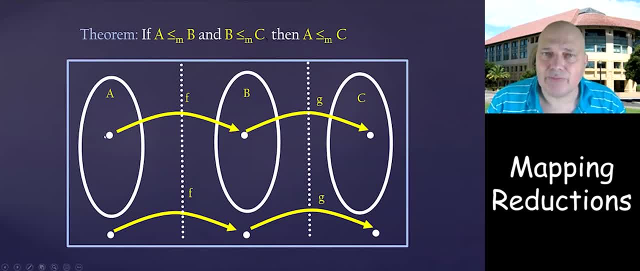 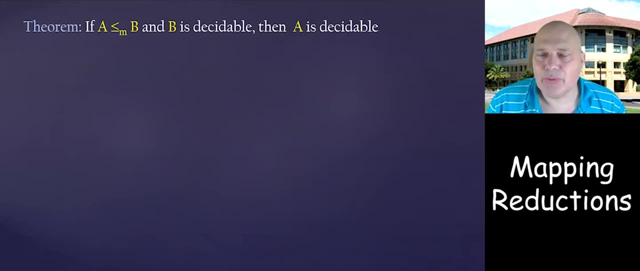 computable. and then it will have the property that when you either, if you start in A, you will end up in C, and if you start outside of A, you'll end up outside of C. And now we see how we're going to use it and, as I said, we're 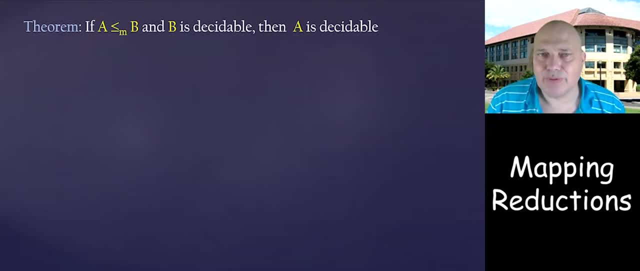 going to use it in the computability or complexity theoretic way of using reductions, kind of in a negative sense. but first let's see the algorithmic sense. So if A is mapping reducible to B and B is decidable, then A is decidable. 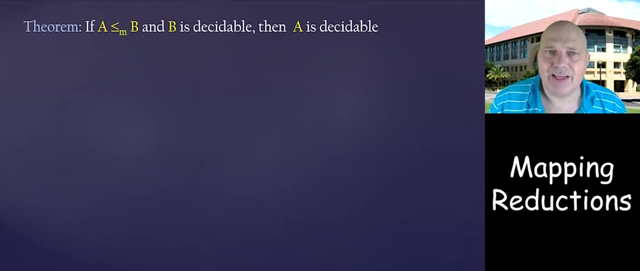 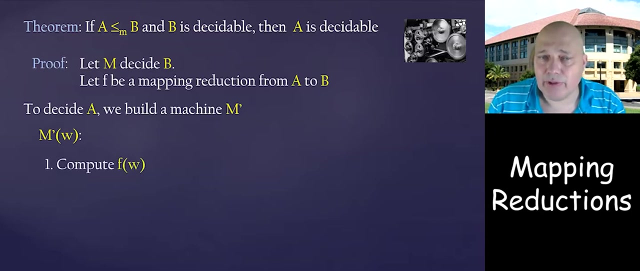 because you can reduce your problem to B To solve A. you can reduce it to B and solve it there. So, and with more details, M decides B and let F be mapping. reduction from A to B To decide A. you can build a machine, M' that first computational F. 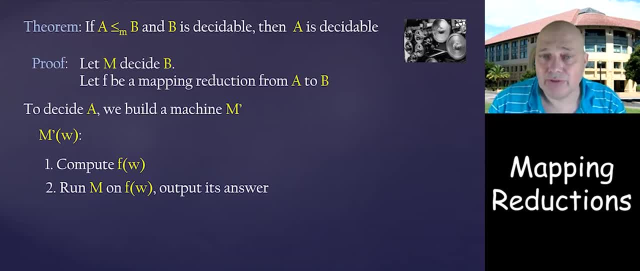 and run M on F and output its answer. So F reduces the problem to B and in. we know how to solve it using M. W is in A, If W is in C, only if f of w is in b. meaning that w is in a, meaning that it implies that f of w. 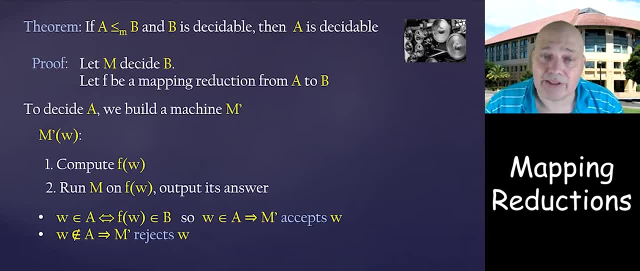 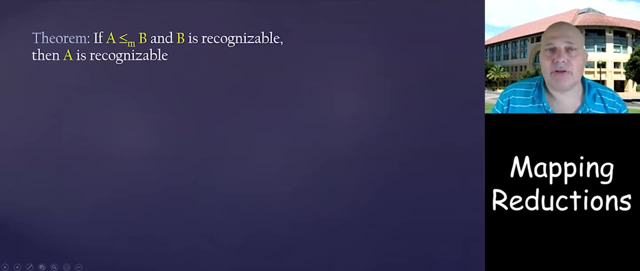 is in b and therefore m prime accepts w. w is not in a means that f of w is not in b, means that m prime is going to reject w. And similarly, if a is mapping reducible to b and b is recognisable, then a is recognisable and the proof is the same proof m recognises. 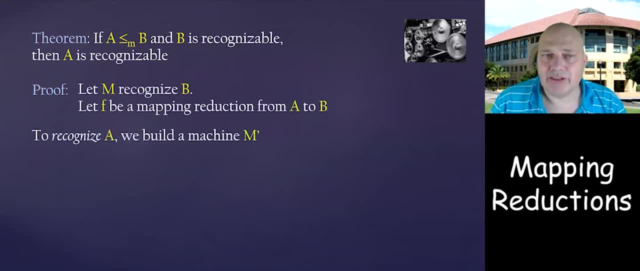 b. f is the mapping reduction from a to b To recognise a. we build a machine, m prime, just as before. You compute f of w, You run m on f of w and output it answers if you get it. So the reason you don't get something that decides is because m doesn't necessarily. 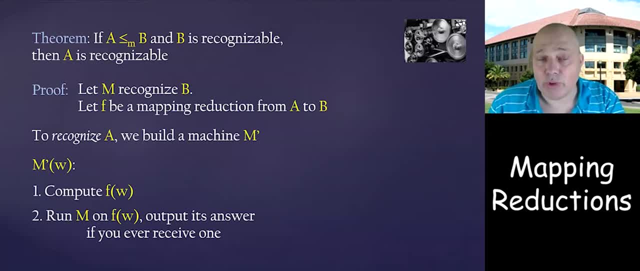 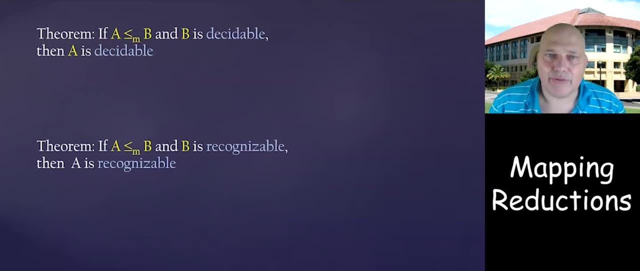 decide: run forever. In that case M prime would run forever, But whenever M is going to halt, it's going to give you the right answer. So these are the two positive ways. If you have a reduction, you can deduce the decidability of A or the recognizability of A from those. 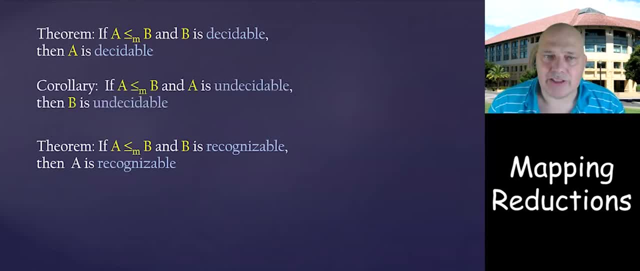 of B. The counterpositive is, the corollaries are that if A is mapping reducible to B and A is undecidable, then B is undecidable, Because if B was decidable, then A would be decidable, And similarly, if A is unrecognizable, then B is unrecognizable. So in this sense, 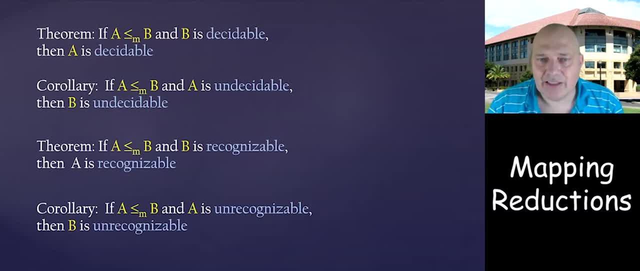 A gives us a lower bound on the difficulty of B And B gives an upper bound on the difficulty of A. So if B is decidable or recognisable, we can deduce it for A, And if A is not decidable or not recognisable, we can deduce it to B. Let's go back to the proof that halting is. 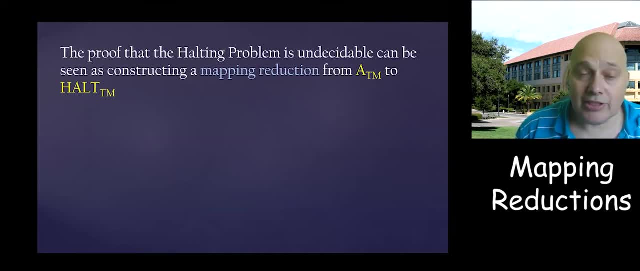 not reducible And we didn't present it this way. but we can show how it can imply a mapping reduction from ATM to HALTM. So we can reconstruct this proof and show a mapping reduction from ATM to HALTM And that would show that HALTM is not decidable. 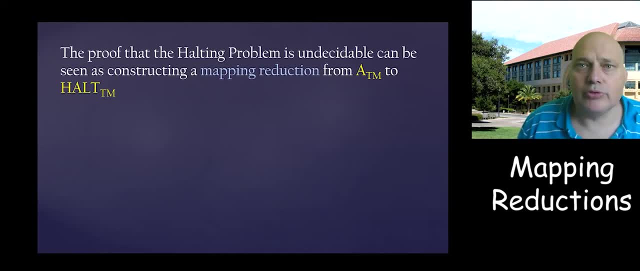 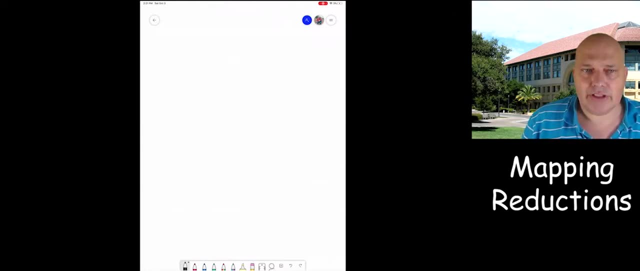 And so for that let me go to the board. So we want to show again that HALTM is not decidable And we will show it by showing a theorem that ATM is mapping reducible to HALTM. And I'm doing it, I'll do a few of those and I'll try to do it slowly, so you 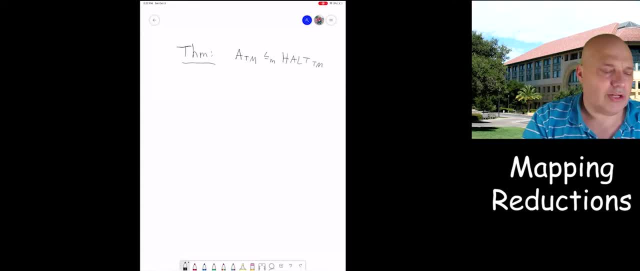 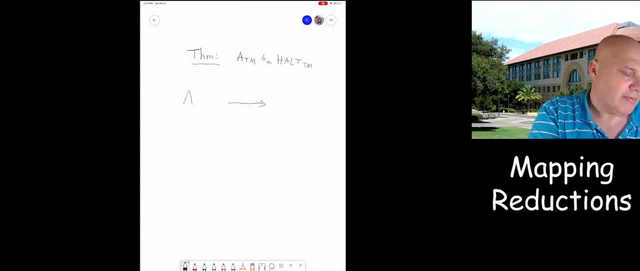 in this direction, from ATM to HALTM, And the first thing we need to do is: syntactically, what does it mean? So we want a function from these inputs to these outputs. we need to ask ourselves: what are the inputs? How do the inputs for ATM look like? So the input? 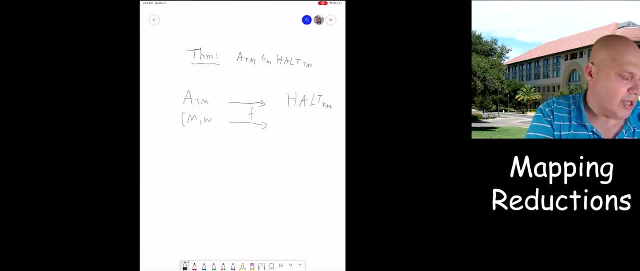 for ATM, let's say, look like M- W And an input for HALT-EM is again a machine and input M prime and W prime. And now we want to ask ourselves what does this proof has to needs to do? 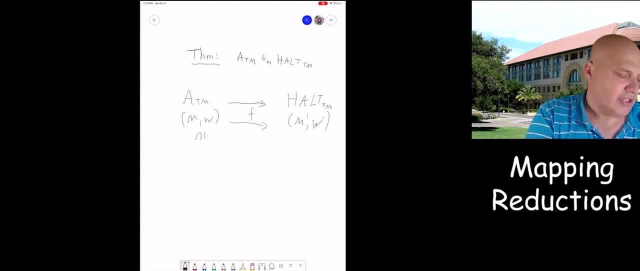 So we need to have that. M? W is in ATM If, and only if, M prime W prime. sorry, so it is in ATM if, and only if, M prime W prime is in HALT. So let's continue parsing it. 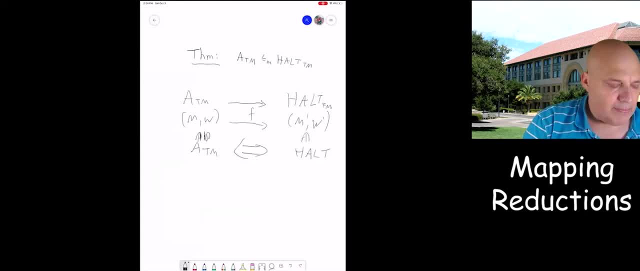 What does it mean that M W is in ATM? It means that M on W accepts. And what does it mean that M prime, W prime is in HALT? It means that M prime on W prime HALT. Now let's construct this M prime and W prime. 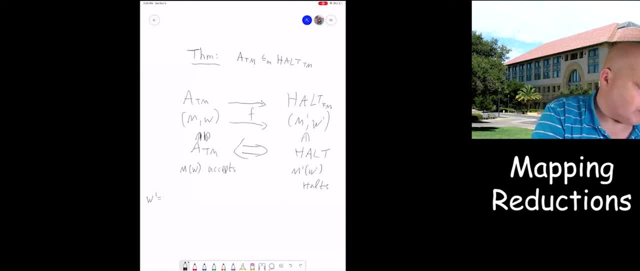 So the way we construct it will first to say the W prime. M prime equals W And we're going to create this M prime, not very different than we had before M prime, which inside we have M. And the way M prime operates: it gets an input X. 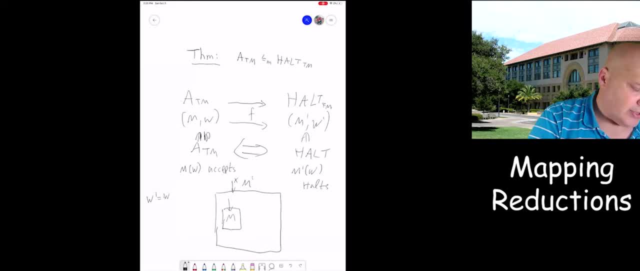 We need to say what to do. We're going to plug X into M. And now, if it is accepting, so it can either accept or reject, If it is accept, we're going to accept. If it rejects, we're not going to reject. 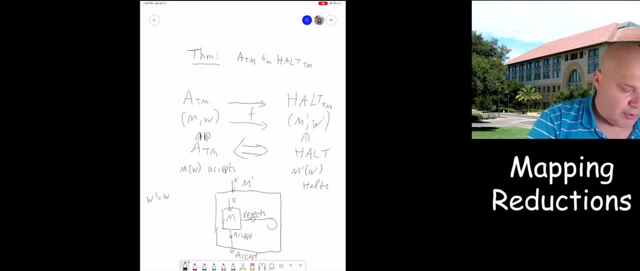 We're going to loop, So we just going to implement some other machine that never HALT, For example a machine that just counts from one to infinity, So just promotes a counter. And of course M can also not HALT. but in this case 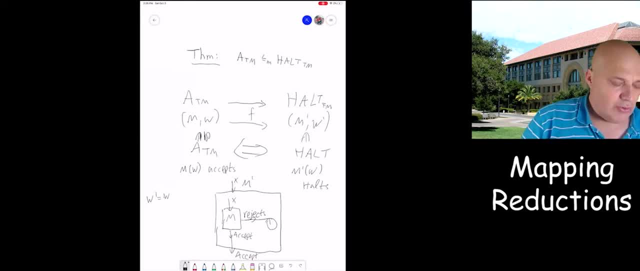 M doesn't, M prime doesn't HALT. So now I want to claim that this construction works, Meaning that I want to say that we have this, this relation: M? W is in ATM if, and only if, M prime, W prime is in HALT. 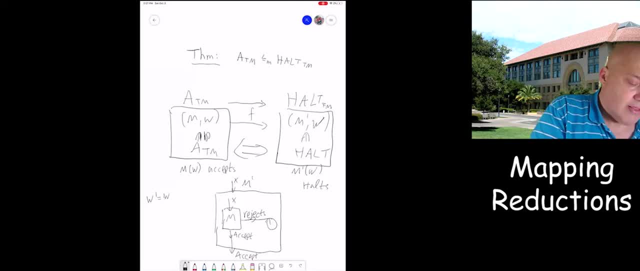 and W prime is W, So let's write it like this: So let's ask: if M W is in ATM means that M of W accepts. So if we plug here: W, M of W accepts, w m accepts and then m prime accepts. 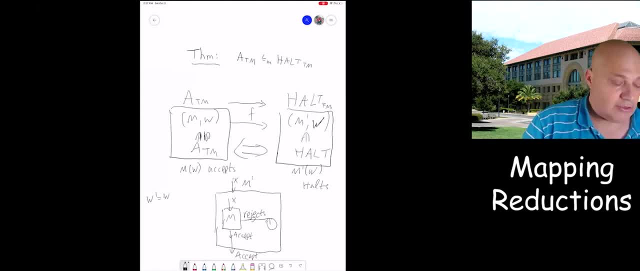 m prime accepts, in particular it halts. So if m accepts, m prime halts. If m reject, then m prime is not going to halt. And if m doesn't halt, which again it means it doesn't accept, then m prime doesn't halt. 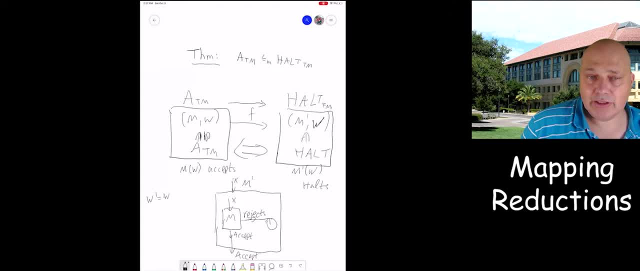 So with this we completed the proof. So we have that m w is in atm if, and only if, m prime w is in halt, And that's a construction we wanted. So we have that atm is mapping reducible to halt m. 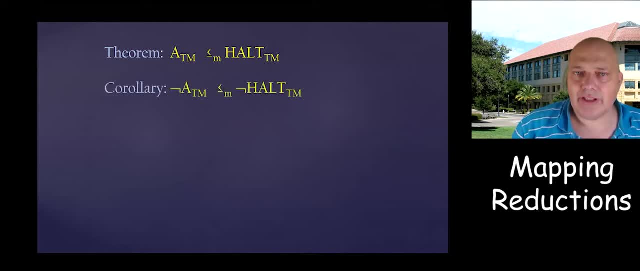 And as a corollary, we will have that not atm is mapping reducible to halt m. So why is this true? Try to think about it for a minute. Well, it is true because any mapping reduction from a to b is also a mapping reduction. 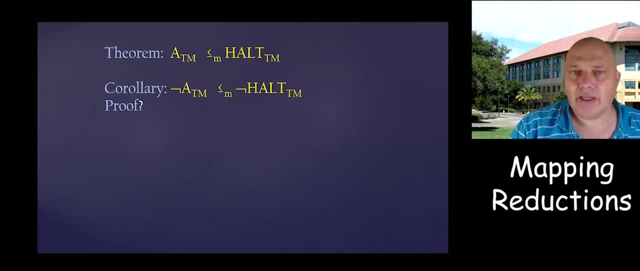 from not a to not b. You can try to convince yourself. The same mapping reduction from atm to halt m is also a mapping reduction from not atm to not halt m. The corollary is that not atm is unrecognizable. Of course we could have also deduced it. 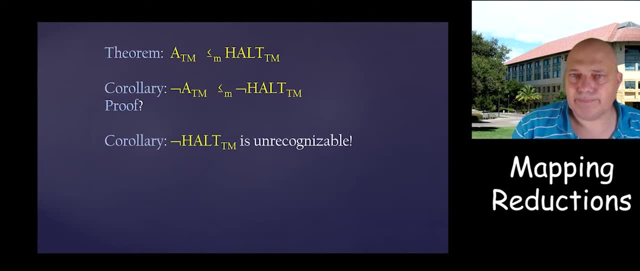 just from the fact that atm is not decidable but recognizable. But the reduction gives us a different way of showing it. Not atm was recognizable then not atm would also be recognizable. And now I want to show the other direction. We want to show that halt m is mapping reducible to atm. 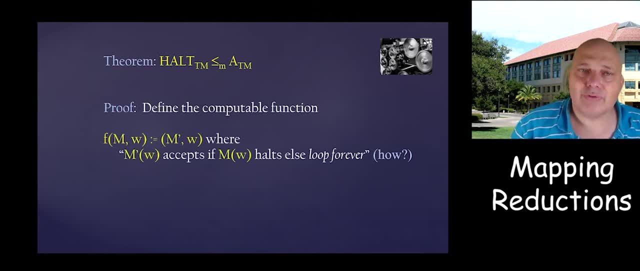 So here we will also have kind of a reduction from inputs to halt m to inputs to atm, And again we will keep the same w. So we will. And we will keep the same w, And we just revise M. So we're going to transform MW to M, prime W. 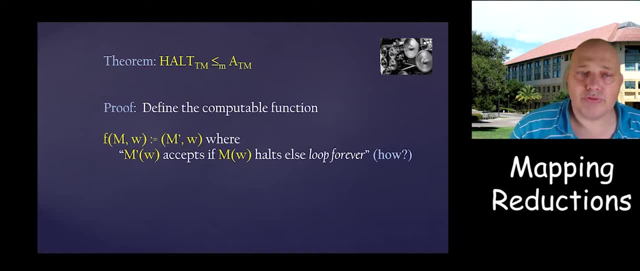 This is the computable function we're going to compute, to define, And the property is that M prime W accepts if MW halts And halts, it loops forever. So think for a second: how can you define M prime in such a way? 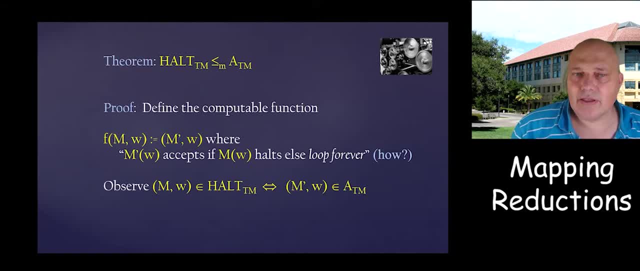 And if that's the case, if we can show such a reduction, then we'll have that MW is in alt M if, and only if, M prime W is in A T, M and we get the construction we wanted. So how would we? I'll give a hint about how to construct this. 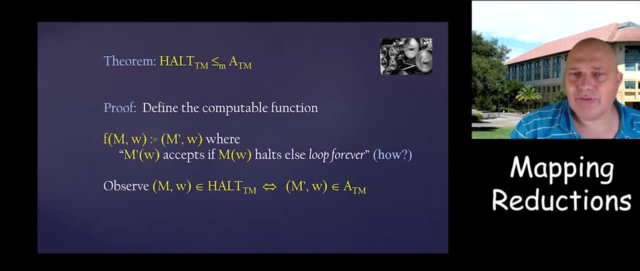 M prime. so M prime needs to accept if M of W halts and else run forever. This is even easier than before. M prime would simulate M on W or on the same input. If the machine halts it is going to accept. 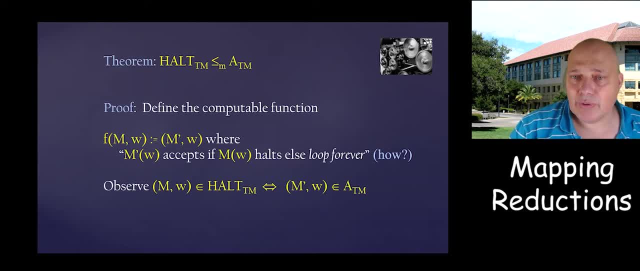 So instead of we're going to ignore what M does The moment it halts and want to output either accept or reject, we'll move to an accept state And otherwise it's not going to halt And therefore our simulation is not going to halt either. 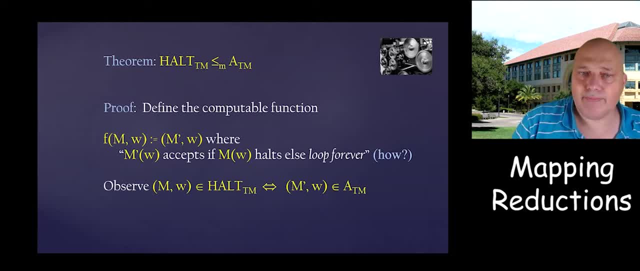 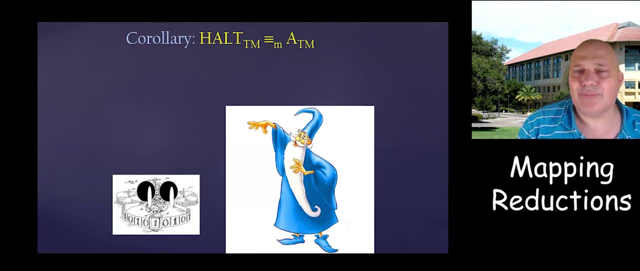 meaning that M prime is not even going to accept. So essentially what we've seen is a reduction from halting M to A, T, M and vice versa. So they are mapping reducible equivalent and these two problems. So if kind of a. 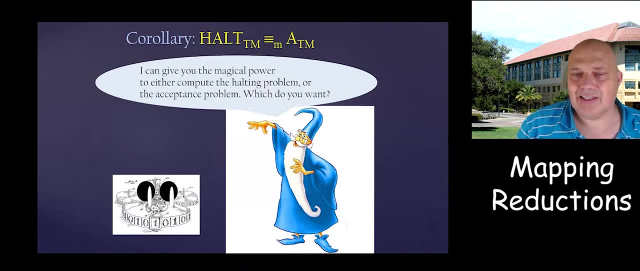 we can imagine a Turing machine. and this Marlin tells the Turing machine: you know, I can give you some magical power that other Turing machines don't have, And the power either to compute the halting problem or to compute the acceptance problem. Which do you want? 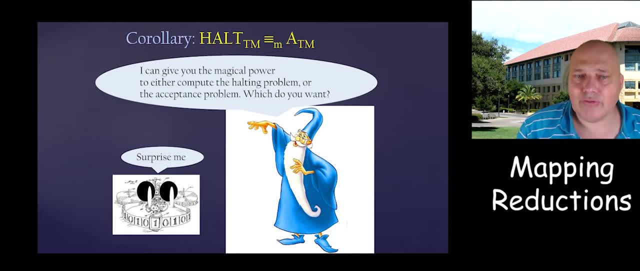 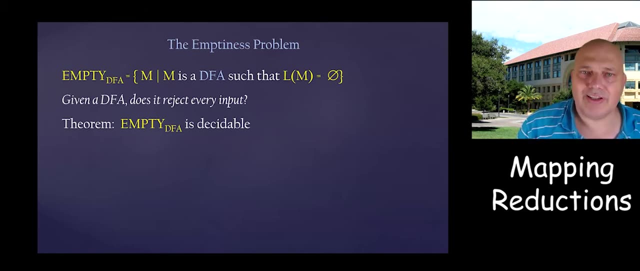 And then the Turing machine has no reason to prefer one over the other, because you can reduce one to the other. They're equivalent to each other. We're going to see a few more examples and, again, to be able to do it more slowly, 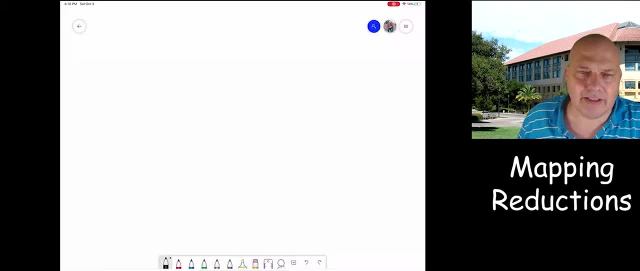 I'm going to go to the board again. The next problem we're going to analyze is the emptiness problem, And we'll see several variants of it, And so the first one is empty DFA. It's M, such that M is a DFA. 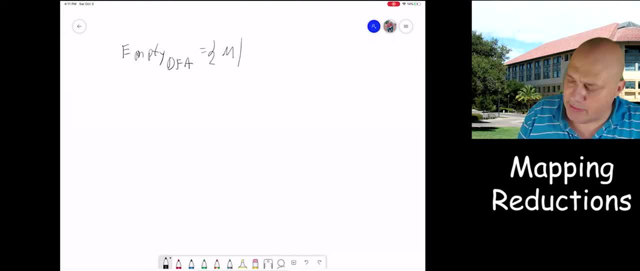 And the language that the M recognizes is empty. So I'm going to write a little bit about the DFA. So there we go. So if I look at the situation, if we look at the cheese score of the cheese score in the basis, 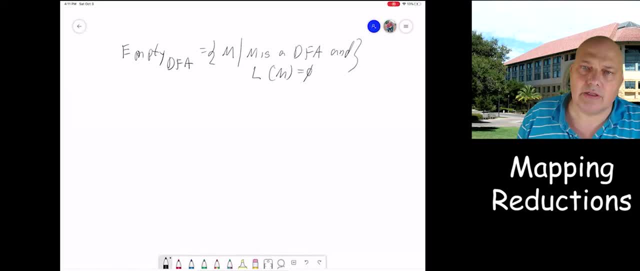 you can see that uh, empty. So M is a DFA and L is empty And the theorem is that empty DFA. so what is it? Is it decidable or not? Yes, it is decidable. And why So empty DFA is? 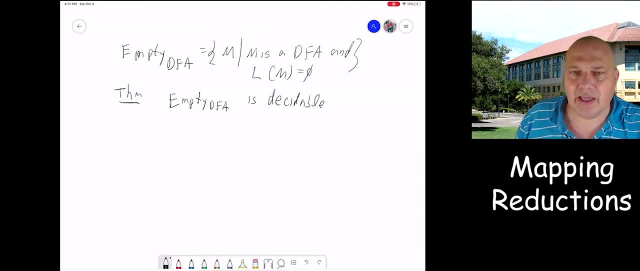 decidable because we can look at the DFA and analyze if there is any accepting state which is reachable. If no accepting state is reachable then we cannot accept anything. But once there is a reachable accepting state then the DFA accepts something in the language It accepts, exactly what allows you to walk on the path from the start to an accepting 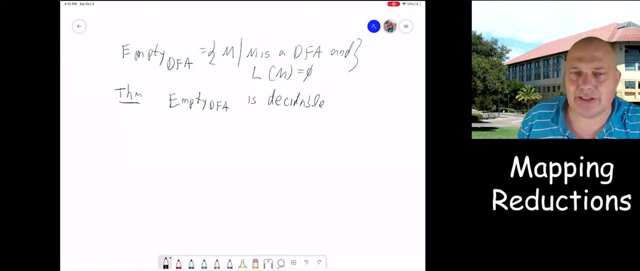 state. How do you verify that there is, that the state is reachable. This is, this is CS161 for you. So there are simple algorithms for connectivity And breadth-first search, depth-first search. you apply any of those and you find if there is any accepting. 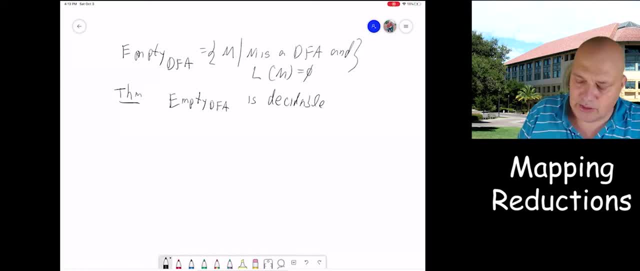 state that is reachable from the start state. So how about empty NFA? Empty NFA is the same, but M now is a non-deterministic, finite automata. Still, L of M is empty. So empty NFA, not surprisingly, is also decidable. You can either directly do the same thing. 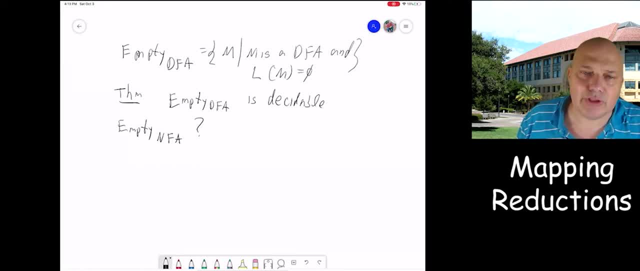 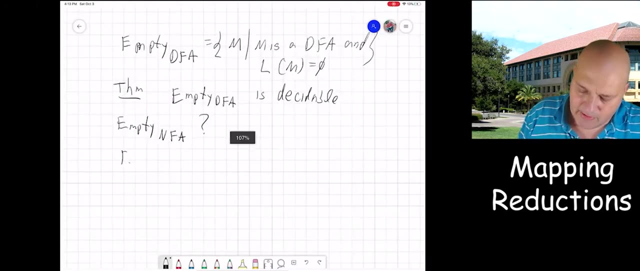 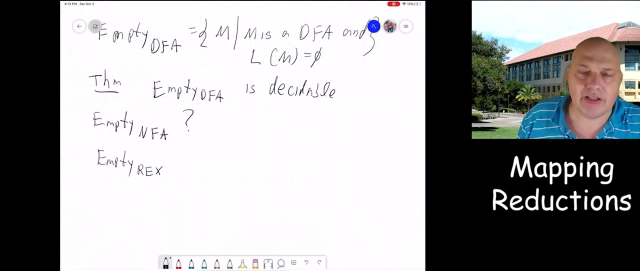 So look for an accept state which is reachable, or reduce the NFA to a DFA and and solve it. solve empty DFA. How about empty regular expression? So here it's the language of R, such that R is a reg, a regular expression, And the language of R is a regular expression. 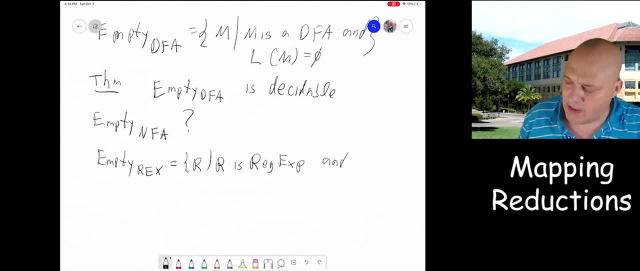 Okay, Okay, Okay, Okay, Okay Okay. The language that it identifies is empty, So is this a decidable? Well, yes, this is decidable, Not surprisingly, for example, because you can turn a regular expression into an NFA and then a DFA and solve it there. 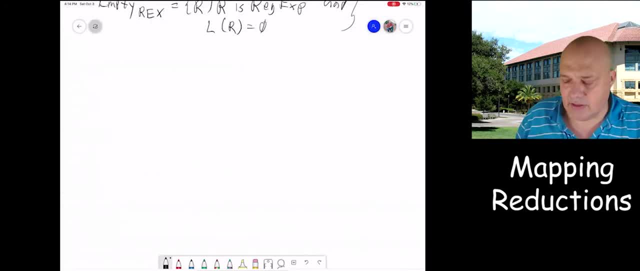 Okay, Okay, Okay, course, empty Turing machine is, as you can expect, M, such that M is a Turing machine and L is empty, Meaning that this program rejects every input or actually doesn't accept any input. So we're asking: is this Turing machine? 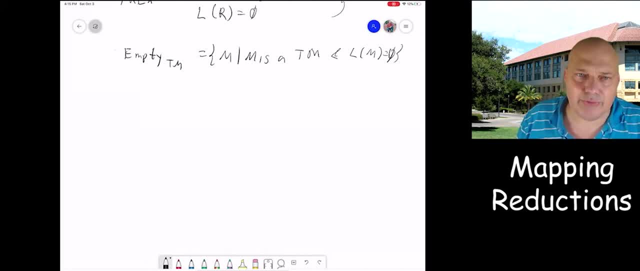 is this a Turing machine that doesn't accept any input? And theorem is so. is it think, is it decidable, is it recognizable? Well, turns out that empty TM is not even recognizable. And now will will prove that So kind of intuitively, or what would we try to? 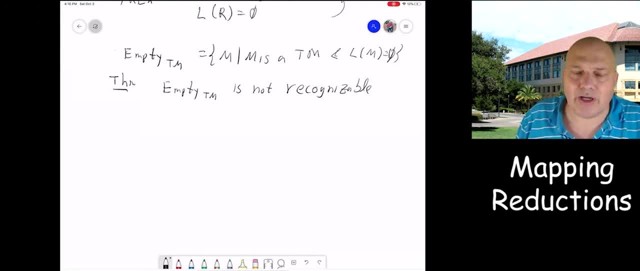 do if we wanted to recognize it, We would try to run it on on all inputs and see if it would be recognizable company. So what we can do here is see that 이 doesn't halt on any of them, But how can we know that you don't halt? You need to simulate and not 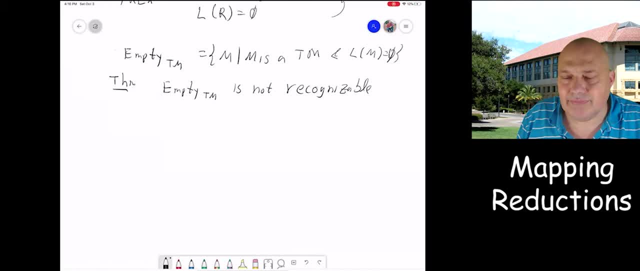 to halt And so kind of intuitively, you'll never be convinced that it doesn't accept anything. Perhaps you just didn't run long enough, But formally what we'll show. so the proof is to show that not ATM is mapping reducible to empty. 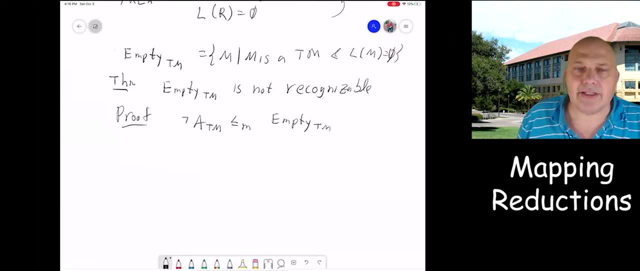 in machine. And since not ATM is not recognisable, then it will tell us that MTTM is not recognisable And that So now we want a function f from inputs of not ATM to inputs of empty. So let's think: what are the inputs of ATM or not ATM? These are pairs M, W. 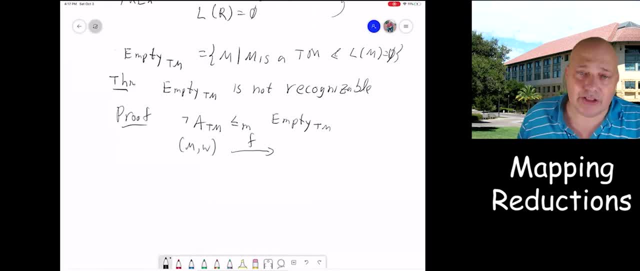 And what is the input of empty? This is just one machine. So, given M and W, we need to transform them to M prime. And what is the property? The property that M W is in, not ATM, if, and only if, M prime is in empty. 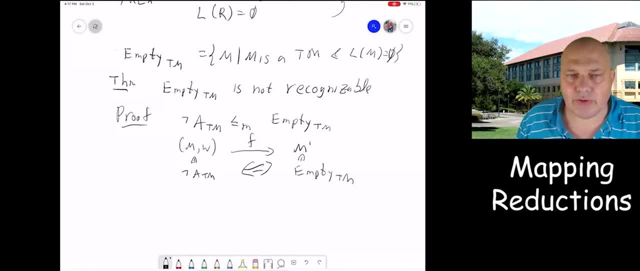 ATM And I do it very slowly. So you see kind of almost mechanically how to do it. At the end there is always something that requires some thought, but quite a lot of thought. A bit of it is mechanical. You just try to see, okay, what kind of inputs, what are the properties. 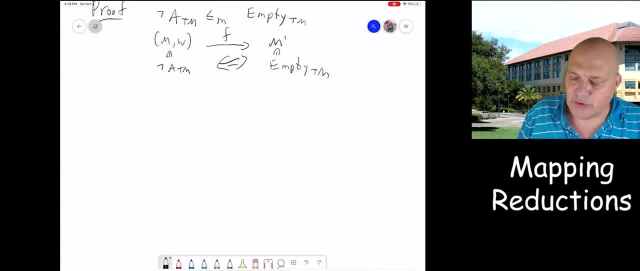 So let's parse that. What does it mean? that not ATM, that M W is not in ATM, It means that M doesn't accept W. If, and only if. what does it mean that M prime is in empty? See, M prime doesn't accept. 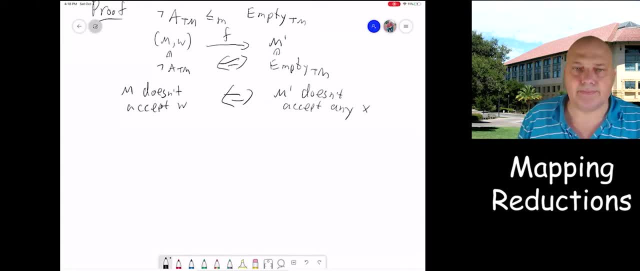 any input: x. Okay, So that's where. so that's as far as we can go automatically, We now know exactly what do we need to transform to. what We need to transform M W to M prime prime, And this is the property that we need. So let's think how we're going. 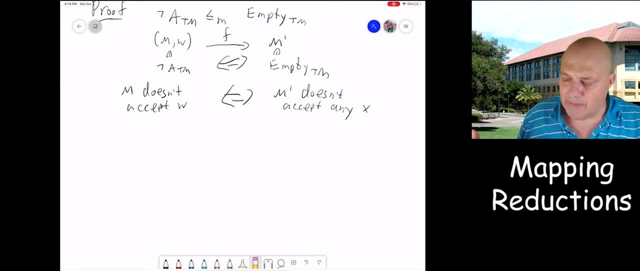 to do it. We know that M prime should accept something as long as M accept W. So the only input we care about, in fact, is W. The way we're going to do it is M prime on X checks if X equals W. It just simulates M on X and 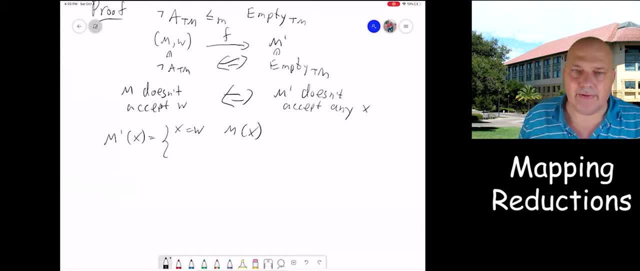 does the same thing as M would do, And if X is not W, then you just reject, You reject outright. So if M doesn't accept W, then N prime would not accept anything, because the only X that it can accept is W And therefore we can conclude the reduction. Okay, so that's. 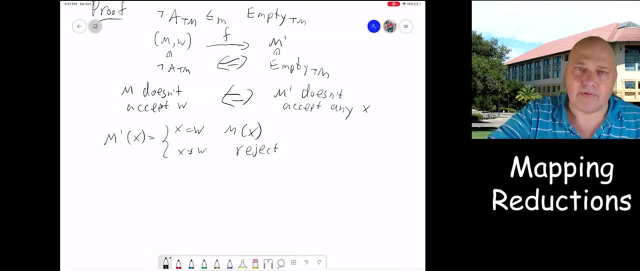 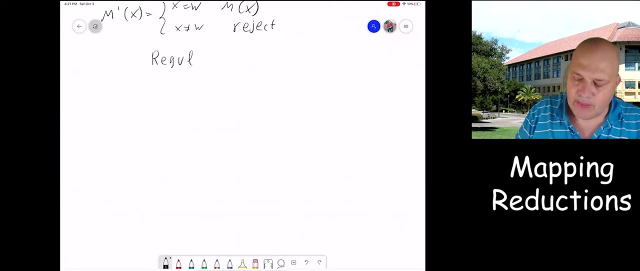 another example. Let's go over to yet another example, Which is the regularity problem, And I'm doing it pretty slowly because if there's one technique I want you to internalize is these reductions, And actually it will become even more important and interesting while we're considering a slow reduction, because 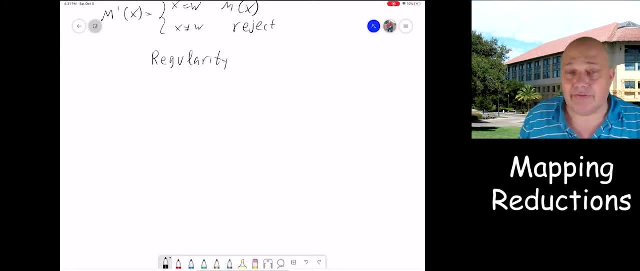 when we talk about efficiency or complexity. So regular- this is the regularity problem. regular Tm are all the Ms such that M is a Turing machine and L of M is regular. So in other words, all the Turing machines such that there is a DFA that would recognize the same problem. 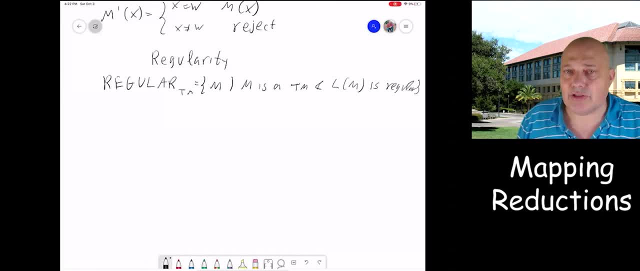 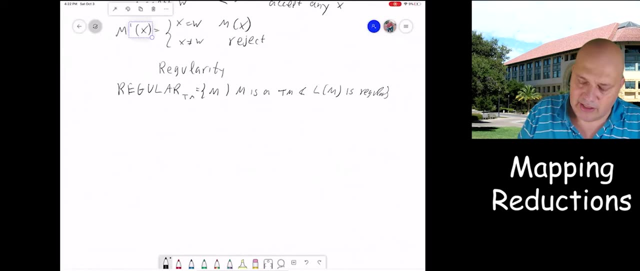 So it's equivalent: all the Turing machines that are equivalent to some DFA. So what do you think? Is it a decidable? Is it recognizable? Is it recognizable? Well, yet again we get that. so the theorem is that regular Tm 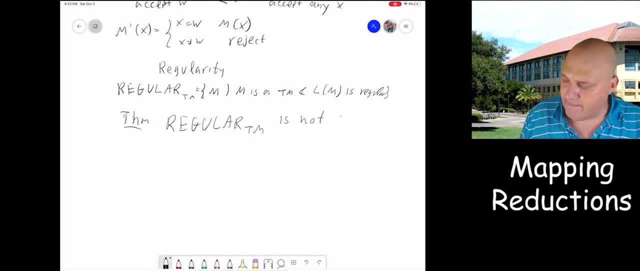 is not even recognizable And by now we have lots of problems to reduce to regular Tm. We could reduce, for example, empty to regular Tm, but the way we'll do it is reduce not a Tm. So we will show that not a Tm is Turing reducible. 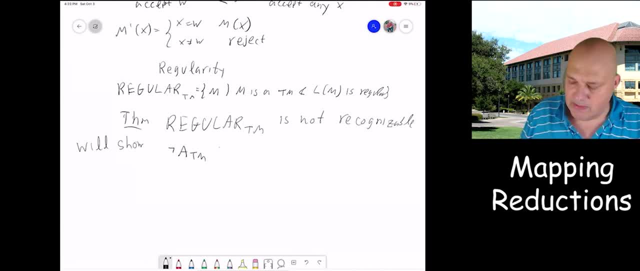 to regular Tm. This is not a bad place to pause and to try to think about the reduction yourself following the what we did before, But now that you're back, let's do it ourselves. So the theory is: if you trapped a T, specified Tm as a D所以. 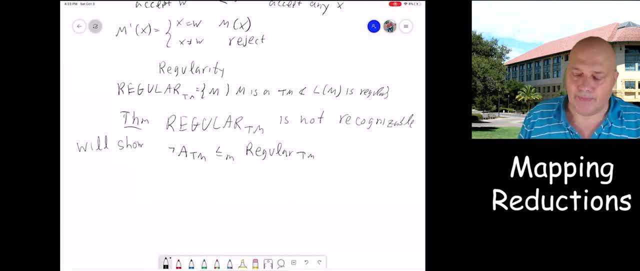 let's not wait late. So it was 1 T, which is minutes about T, which was remaining at the end of the expression. We could then get a bit of variance between them, especially. So what is the input for NOTATM? This is again MW and we need to. 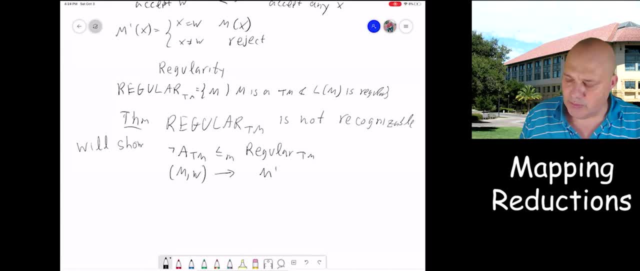 transform it to the input of regular, which is again just one machine, M', and what we need is that MW is in NOTATM if, and only if, M' is in regular TM, meaning that if M doesn't accept W, this will be the case. 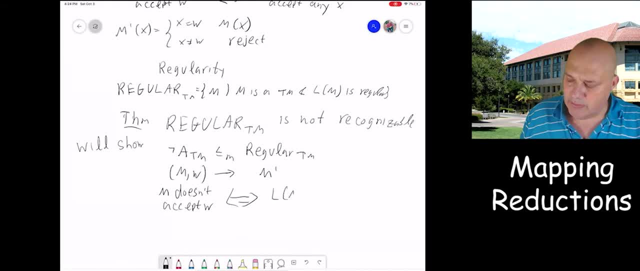 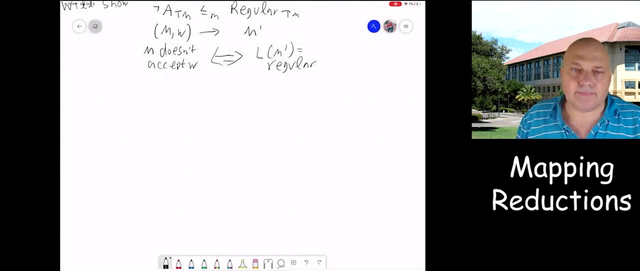 if, and only if, the language at M' except is regular. Okay, so that's the reduction we need to do, and how are we going to do it? and we're going to define M'. it's a little bit similar but slightly more complicated than the, the previous reduction, and so M' on X. 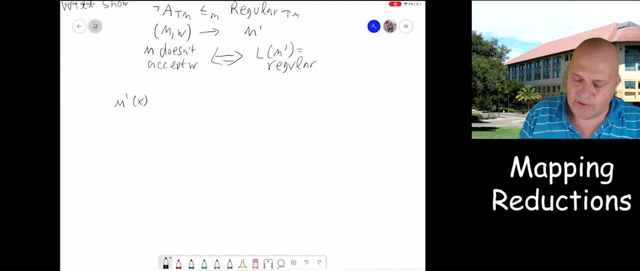 and going to do the following: if X equals 0 to the N, 1 to the N and for some N, then simulate M of W and other else you reject. So what are the two options that can happen? if M' is going to, if M accept W, then M' is going to accept every. 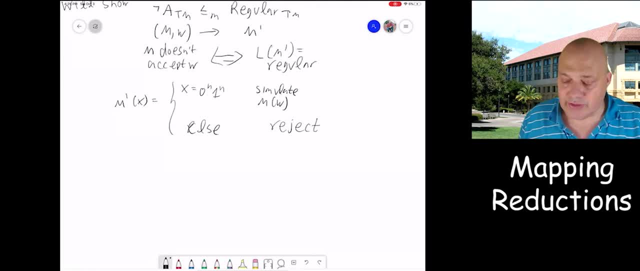 string 0 to the N, 1 to the N, because for every such string, when X is 0 to the N, 1 to the N to the n, we are just going to simulate m on w it's going to accept and therefore, 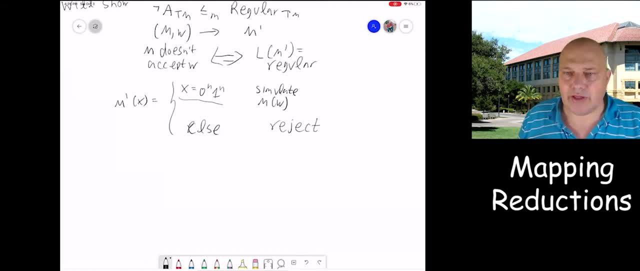 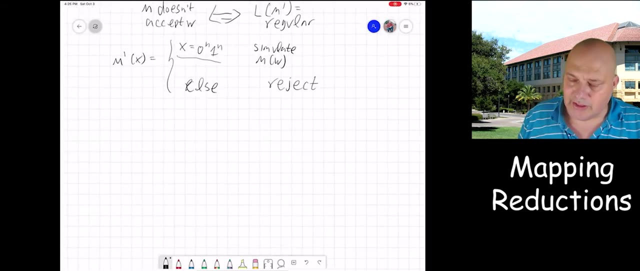 we're going to accept it, Otherwise we're accepting nothing And recall that the empty language is regular, whereas the language that contains 0 to the n, 1 to the n is not regular. So kind of writing it a little bit more slowly if m. 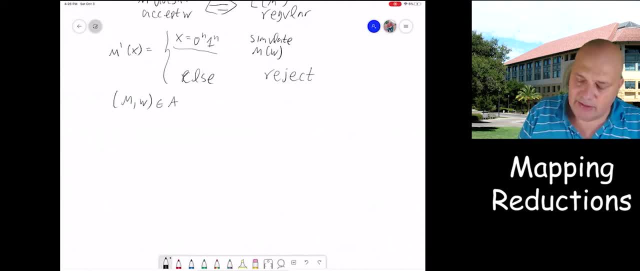 w is in ATM, it implies that m m prime, so L of m prime, is 1 to the n, so 0 to the n, 1 to the n, where n is some natural number Which is not regular. So, alternatively, when m w is not in, not ATM, then we have: 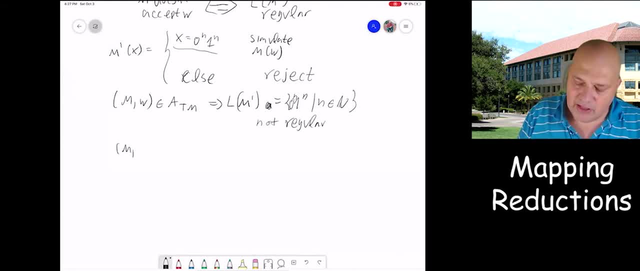 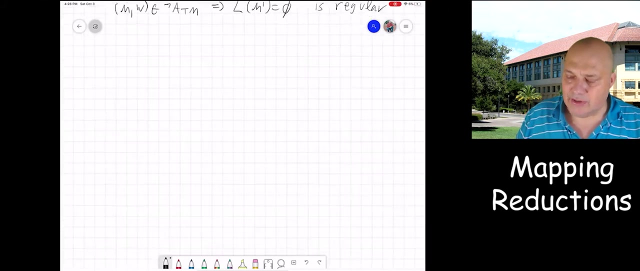 something that's regular. On the other hand, when m w is in, not ATM, then L of m prime is empty. is the empty language which is regular. And this concludes this reduction. We'll give one last example here, which is the equivalence problem. 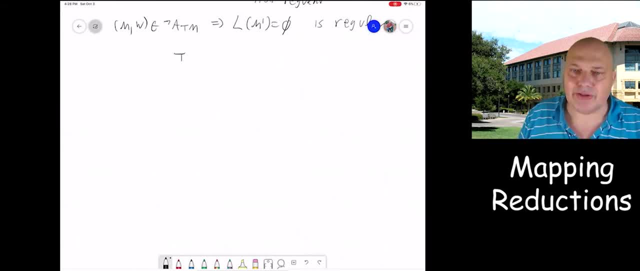 And this problem will actually be interesting. And this problem will actually be interesting later on. So equivalence tm now gives you two machines: m it over pairs m n, such that m and n are Turing machines which accept the same language. So these are equivalent Turing machines. L of m. 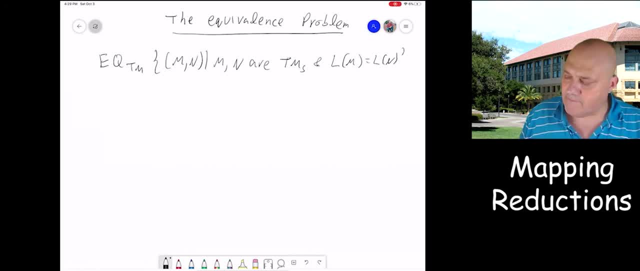 equals L of n. And so when, if we ask the same questions about DSM, we're going to have two DFA's, and then actually we we know how to to compute the equivalence of two DFA's. We can do it by first reducing both of them to to the minimal DFA, and then verifying that the 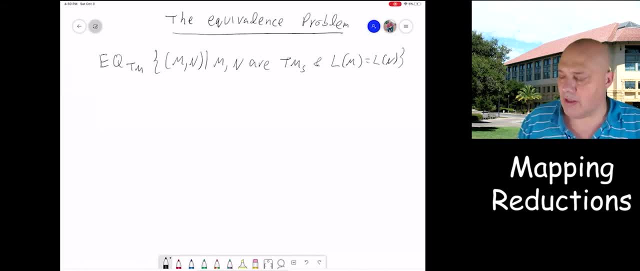 DFA's are equivalent to each other, which we have. all these tools from the previous chapter. But what do you think about this problem? Is it decidable, Is it recognisable? So the theorem is that the equivalence problem for Turing machines is unrecognisable. 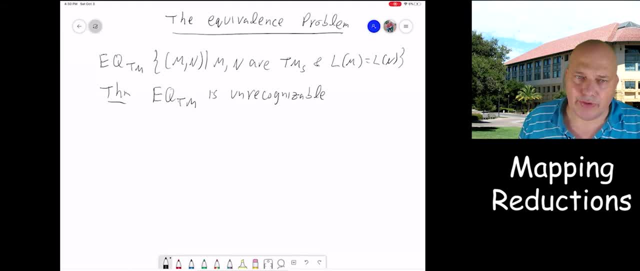 And how do we do that? So, again, by now we have quite a few examples, so we need to choose the one that we are the most happy with, And we'll show that empty Turing machines is mapping reducible to equivalent Turing machine. So again, what we try to do is we're going to have two Turing machines. So again, by now we have quite a few examples, so we need to choose the one that we are the most happy with. So again, by now we have quite a few examples, so we need to choose the one that we are the most happy with. 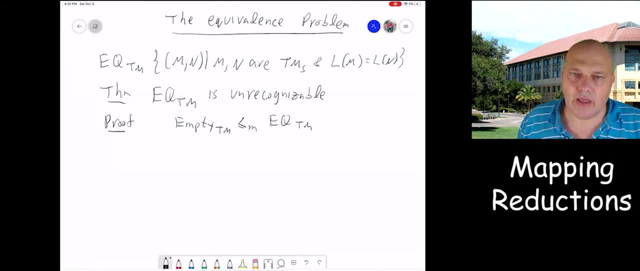 So we need to choose the one that we are the most happy with. So we need to choose the one that we are the most happy with, And then what we're trying to do here is reduce. so we need some function that takes inputs of empty to inputs of eq. 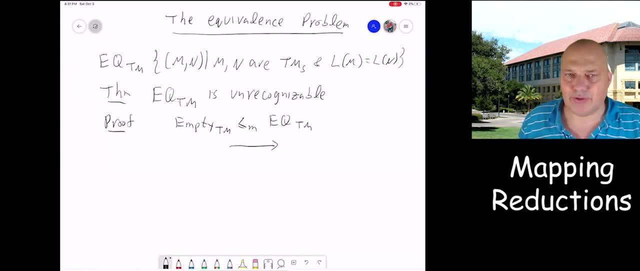 And I'm going to tell you what this reduction is going to look like. The input of empty is sum Turing machine And it's going to get us to the value of Turing to input for equalities tutoring machines. right, It is M and we're going to. 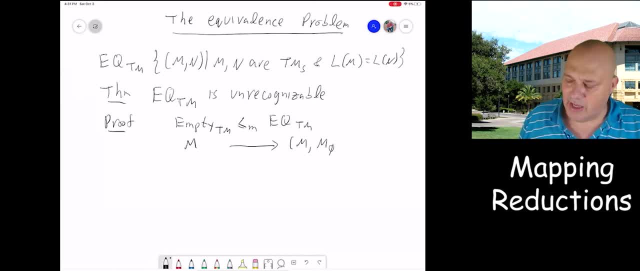 so to have M naught. So this is a reduction where we are actually going to keep one of the ingredients. So M is reduced to M comma, M naught right. The input of equivalence is the same. it's a pair of Turing machines. 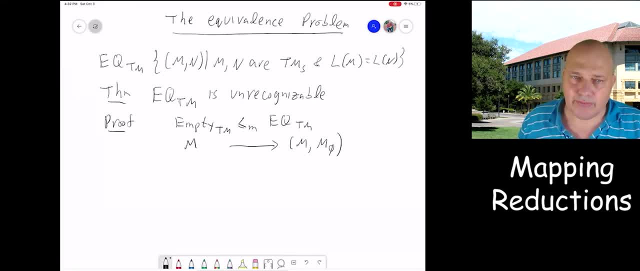 And this reduction is going to be pretty simple. M naught is some so is a dummy Turing machine, and that M naught rejects everything. And so we just have no except states, or except state is disconnected from the start state There is no path from except to start. 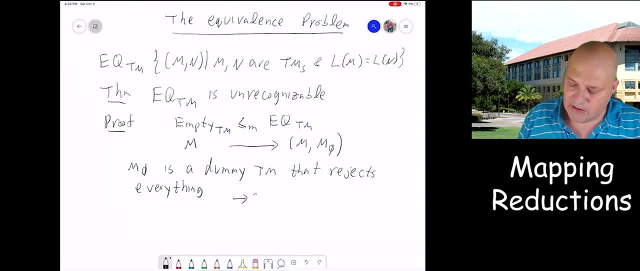 So we can have something like this: This is a start state, this is an except state, and you have all the edges or self loop here and here. So you're just going to start and end it in the start step, which is a reject state. 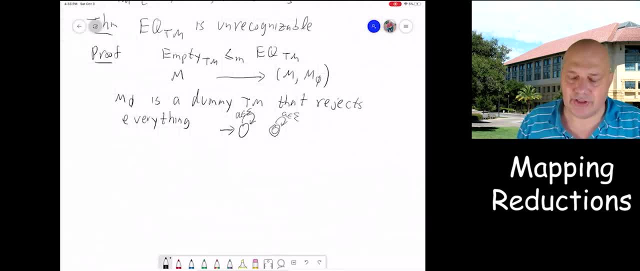 And I wanted to claim that this is a reduction and it's sufficient, Because M is in empty Turing machine If, and only if, just the definition of empty Turing machine L of M is equal to the empty, the empty language, which is just L. 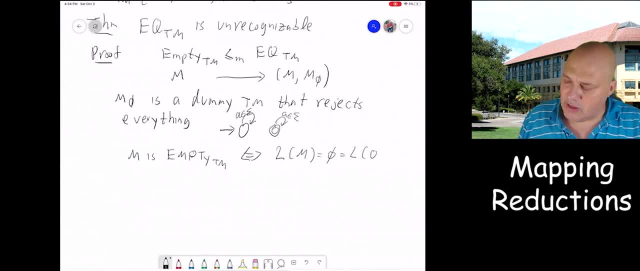 So again, if you can see that this is just an empty Turing machine of L of M- sorry L of M naught, And this is just by definition, if, and only if, M M naught are in equivalent during machine. So that's the last reduction I'm going to. 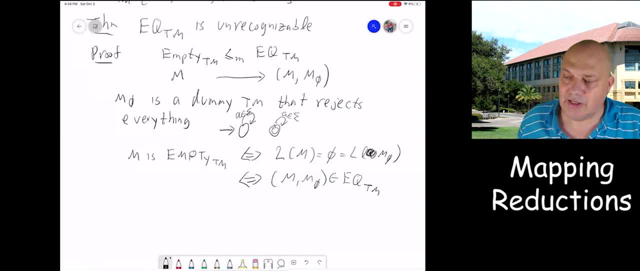 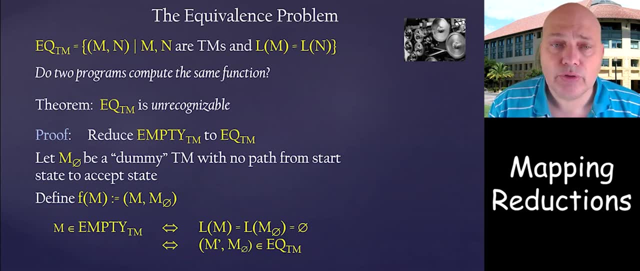 I wanted to do on the board and and with this we'll go back to the slides. So so far we've seen a few reductions: mapping reductions that help us show that problems are not recognizable or not decidable, And the ingredients are. 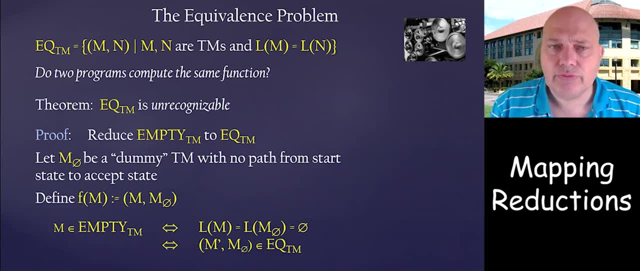 always to to first show a mapping, to argue that the mapping is efficiently computable. We didn't invest too much time in it, but this is one ingredient. you need to argue all the time And then to show an if and non-if that 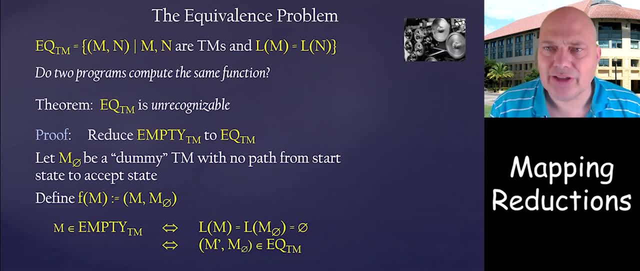 the, the input to the reduction is in the first language. if, and only if, it is in the, the output is in the other language. This is something that's often where people, so the thing that you often will forget is either to show that something is computable, that the 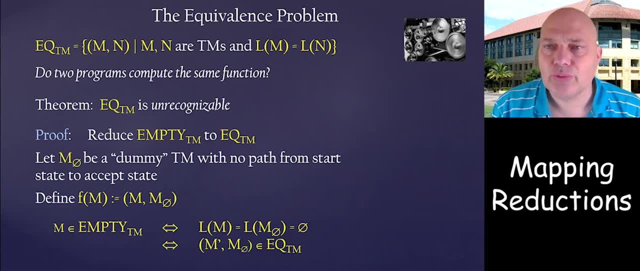 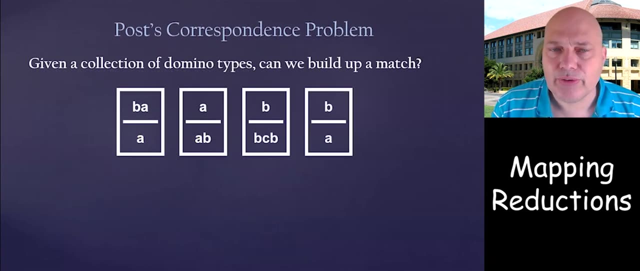 mapping is actually computable, or you'll only show the if and not the only if, or vice versa, you design it to do one side, but you forget to argue about the other side. All of the problems that we discussed were about computation, And I want to. 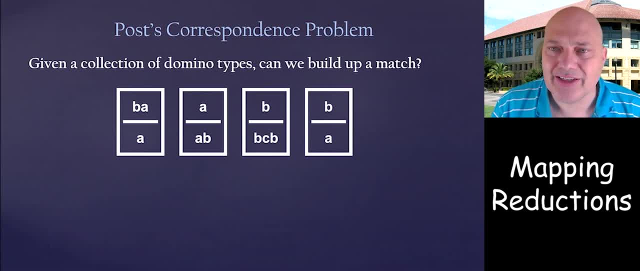 give you a sense that not all problems look like or directly apply to computations. So here is another problem, the post-correspondence problem, and, and in this problem the input is, or collection of domino types and like we see here and you want to compose them. 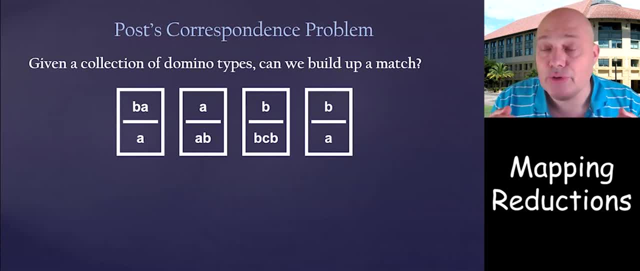 in some order and you can reuse and domino domino types as many times as you want, such that the string on the top will equal the string on the bottom. so here, if we take the first two and then we live on the top BAA and on the bottom 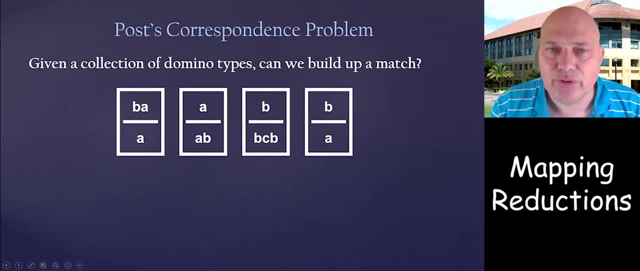 AAB, and this is, of course, not a match, but if we first use this one and then use the first one, then we will have ABA on the top and ABA on the bottom. this is, of course, a very short sequence and in general the sequence can be large and 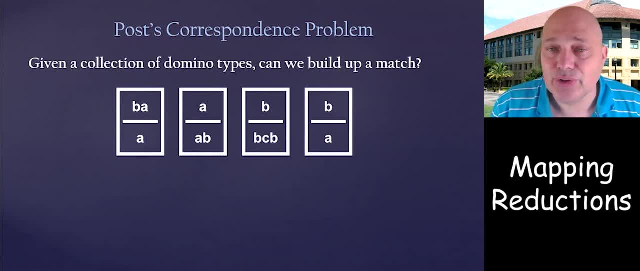 you cannot and you can reuse domino, so there is no way to just exhaustively change the sequence. Check all combinations. this is the problem. P is in PCP. this is, by the way, not the most interesting PCP I think that we will encounter in this course. 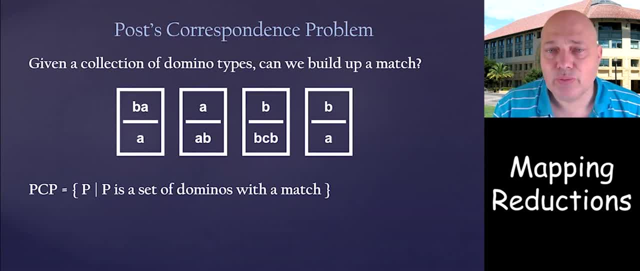 such that P is a set of dominoes with a match and turns out that PCP is undecidable. and the proof. I'm not going to talk about the proof. the proof is in sipser and I think it's a reduction perhaps from ATM and what this shows is: